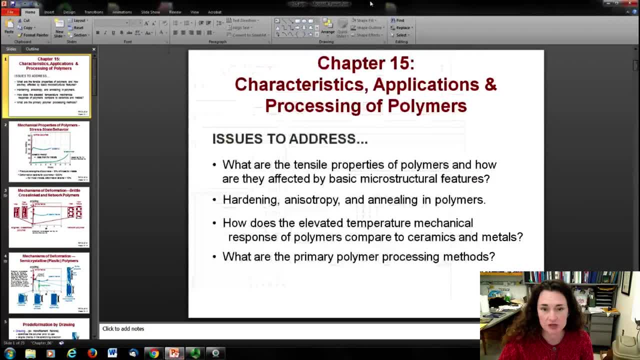 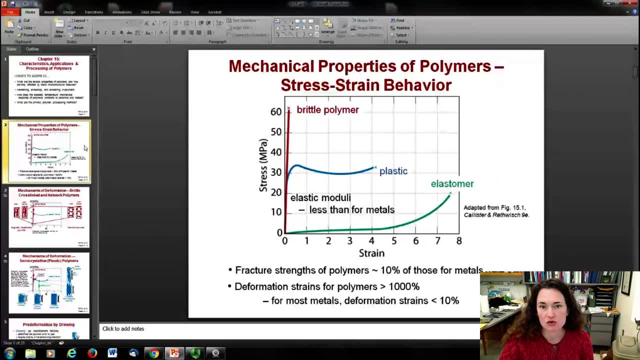 Hi. so today we're going to be talking about Chapter 15, which is Characteristics, Applications and Processing of Polymers. So the stress-strain curves, talking about the mechanical properties of polymers. the stress-strain curves for polymers can vary a lot. 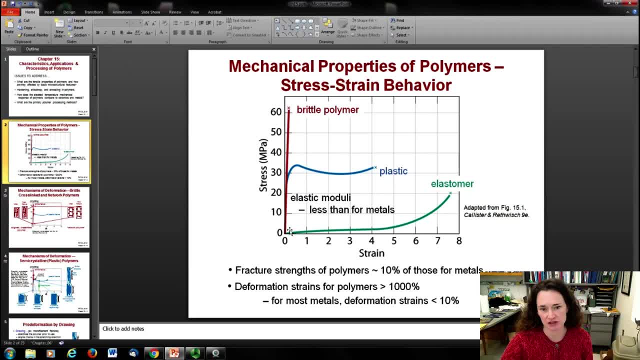 So you can have a stress-strain curve that looks very similar to what you would see for a ceramic, and those are your brittle or glassy polymers. You can have a stress-strain curve that looks a little bit more similar to what you might see for a metal and that's kind of your plastic polymers. 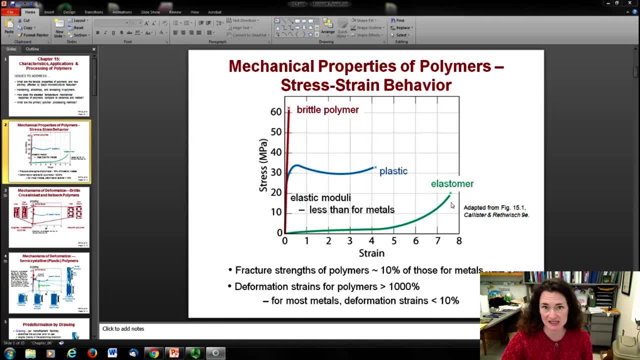 And then you can have the stress-strain curve for materials called elastomers. When I think of elastomers, I think of rubber bands, And they're very unlike both ceramics and metals. You can see, the stress-strain curve looks very, very different from what you would see for a metal or a ceramic material. 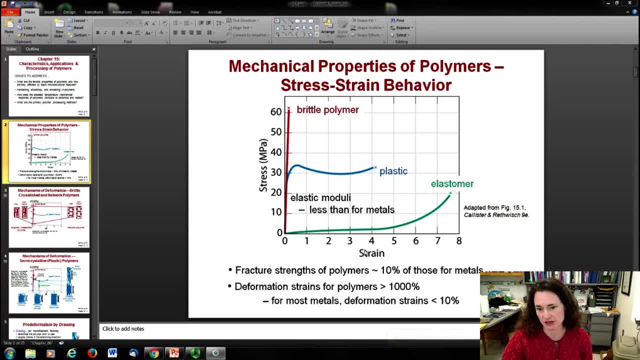 For all polymers the fracture strength is going to be a lot lower- about 10% of the time- But of course they're going to be a lot more elastic. They're going to deform a lot more than a metal. You can have the elastics or the ductility or elasticity of a polymer be a thousand percent or more of what you would see for a metal material. 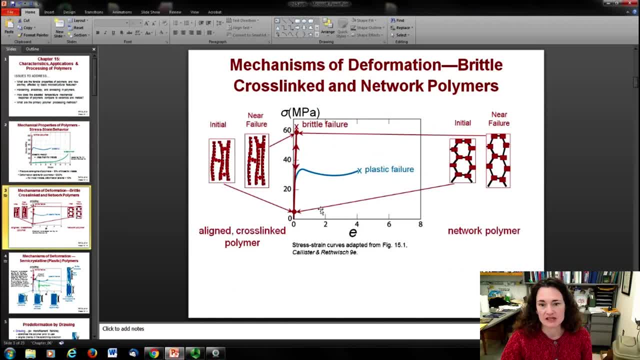 Now let's look at the brittle fracture and the plastic failure. First of all, the definitions of some of these things are a little different for polymers. First of all, the definitions of some of these things are a little different for polymers. 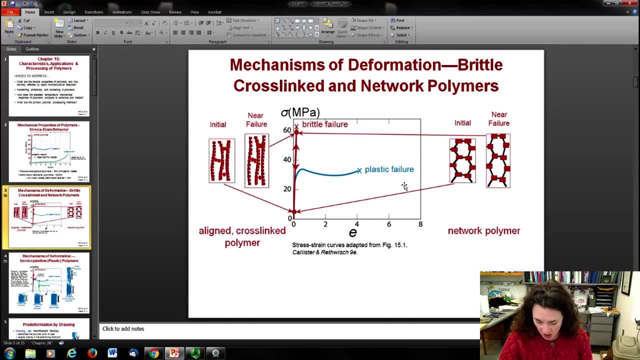 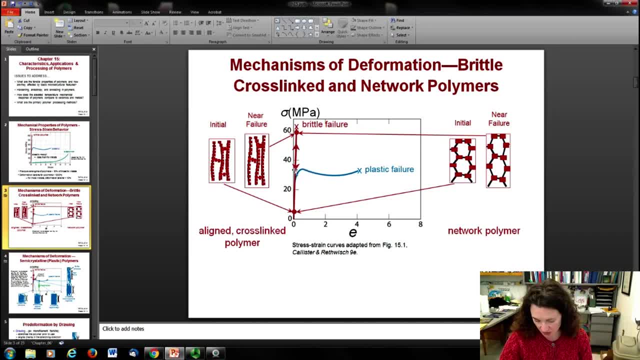 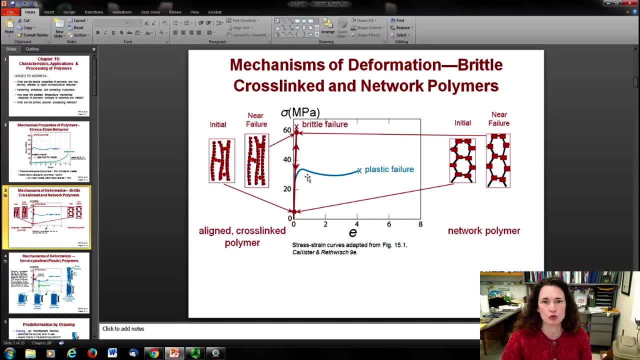 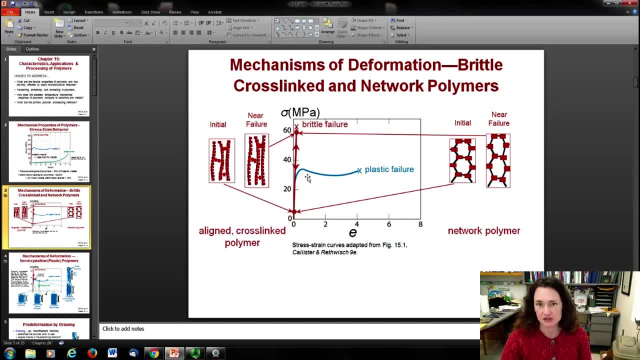 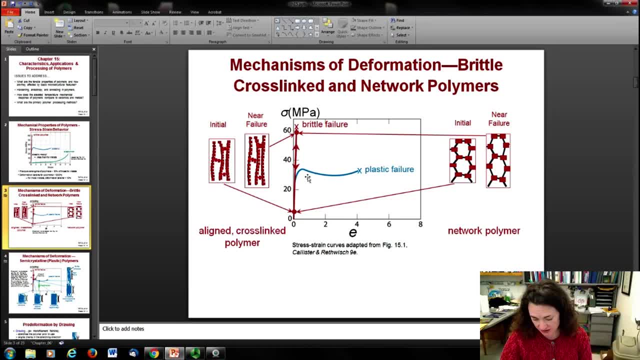 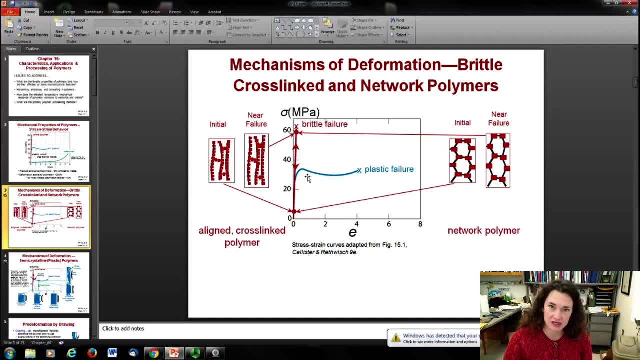 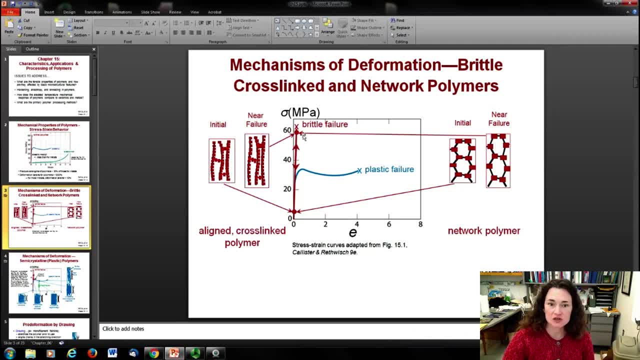 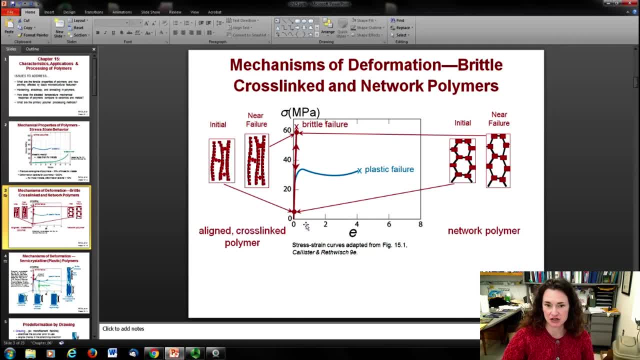 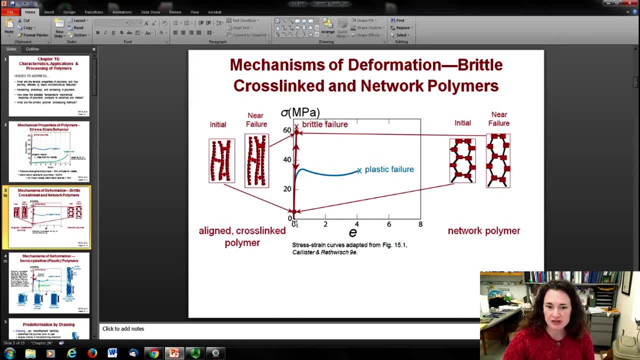 That's different from a metal. remember where the yield strength is defined at, say, a 0.002 strain or 0.2% deformation of the metal. That's different from a metal. remember where the yield strength is defined at, say, a 0.0% deformation of the metal. 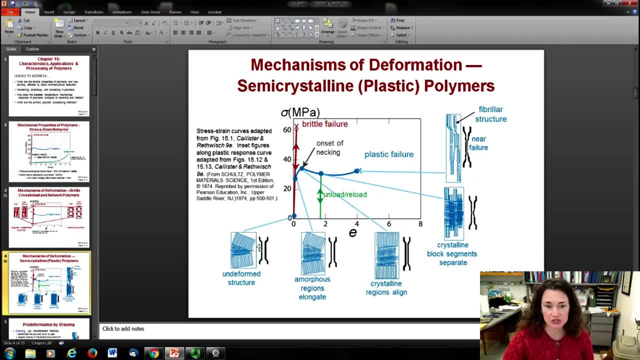 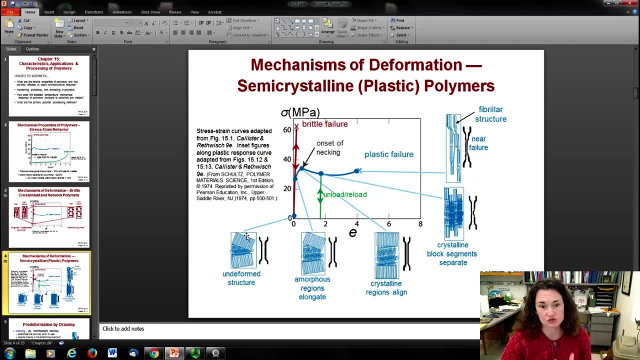 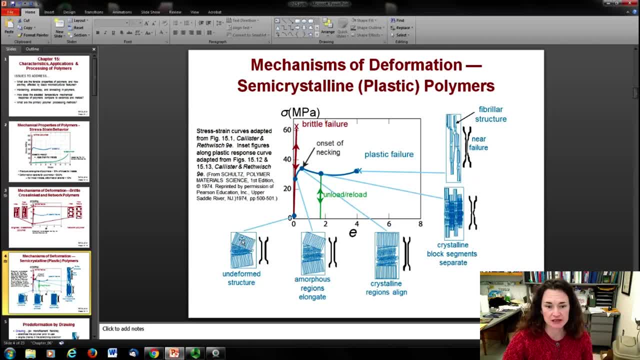 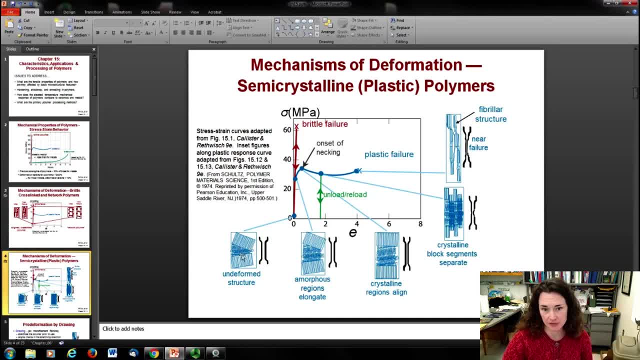 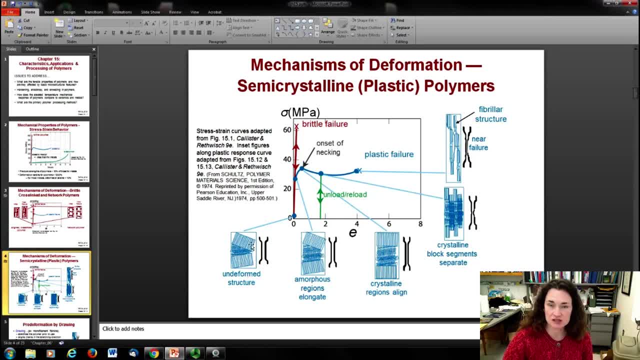 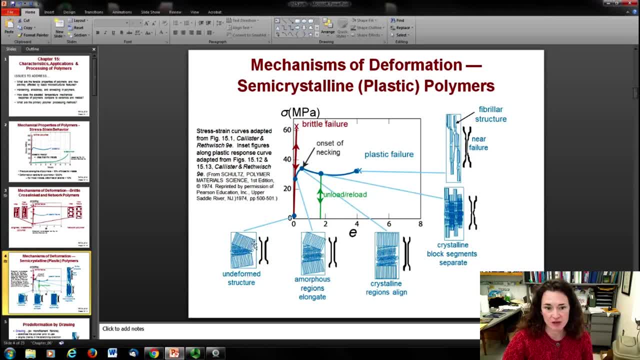 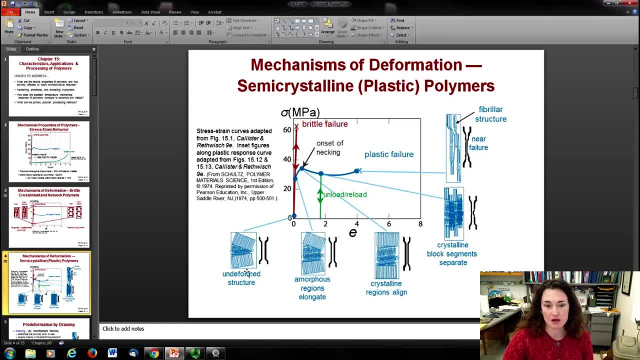 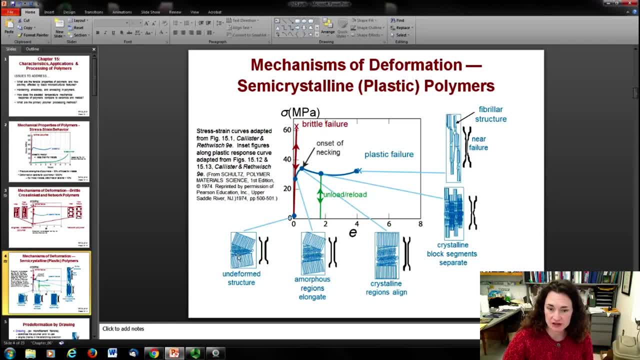 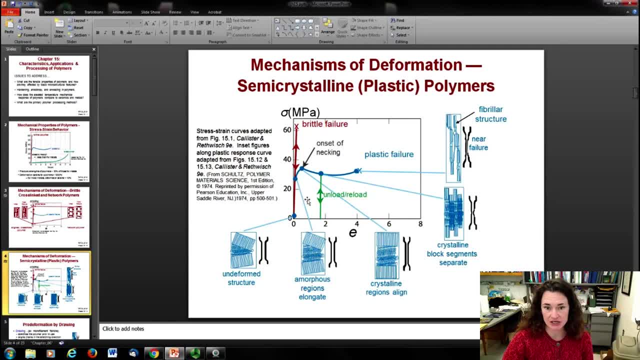 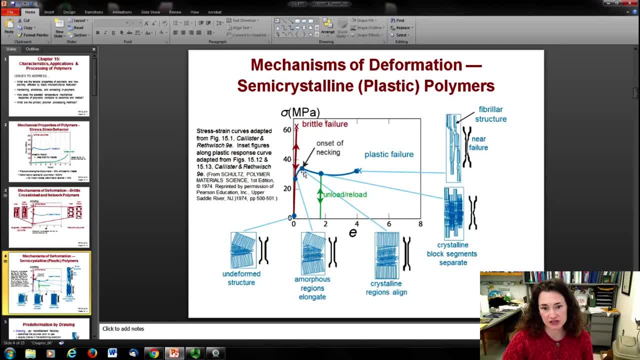 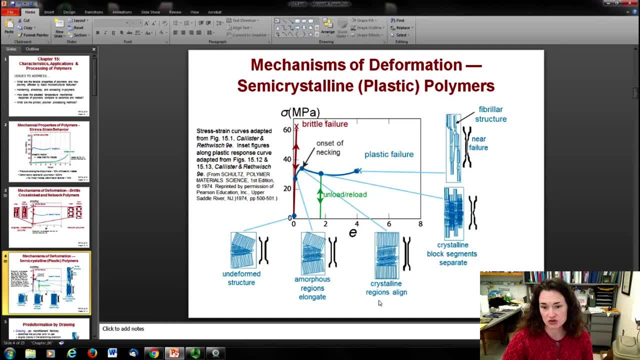 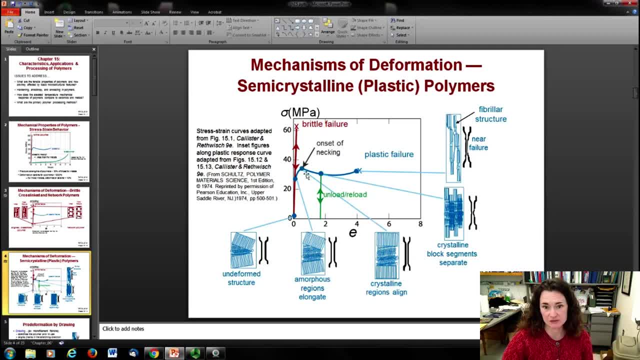 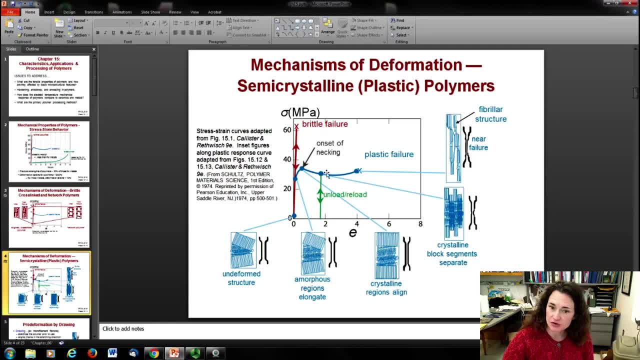 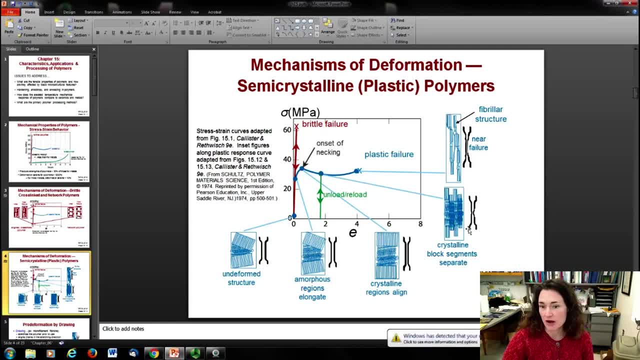 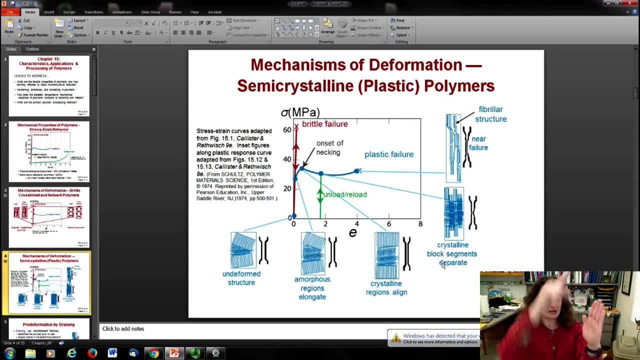 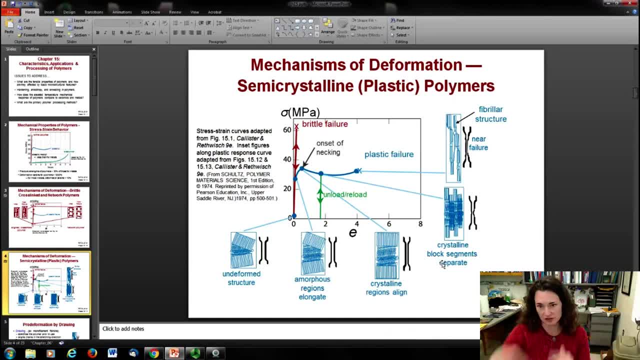 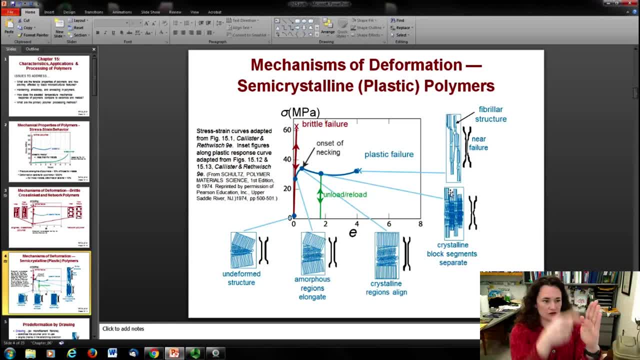 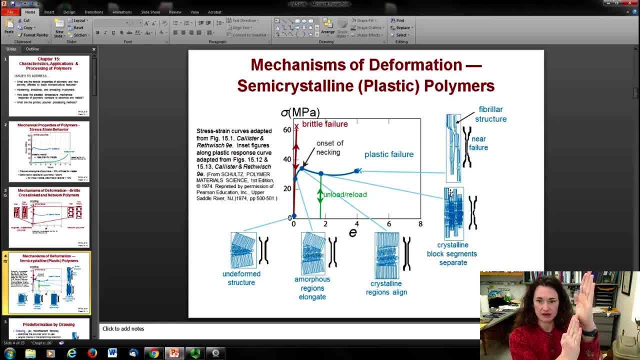 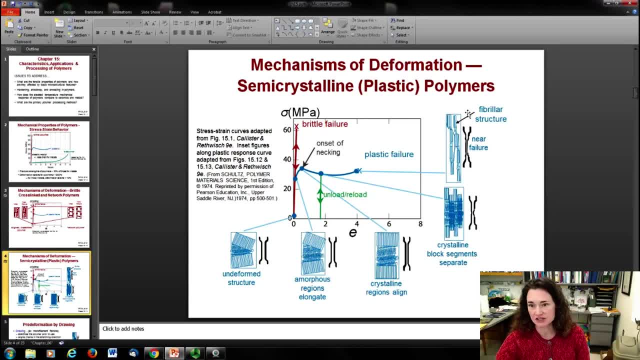 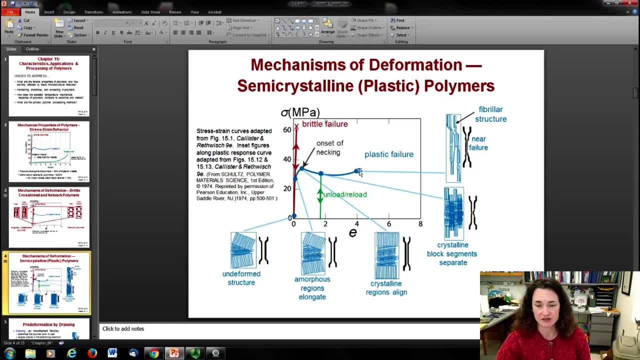 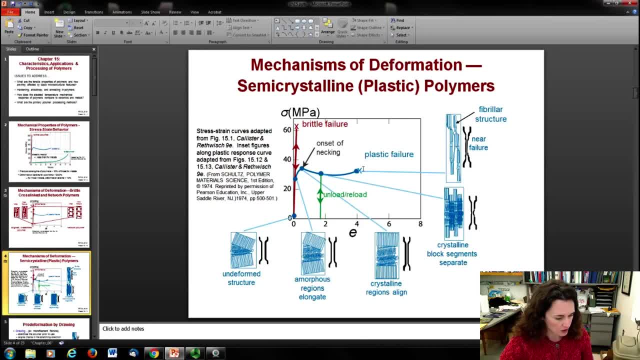 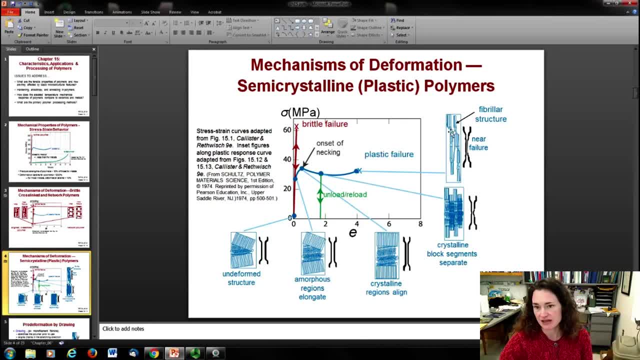 Um, What happens is in this, Um, What happens is in this alignment region. that actually causes strengthening of the polymer right there. It's similar to um, similar to cold working in metals. It can cause a strengthening of the polymer there near failure. 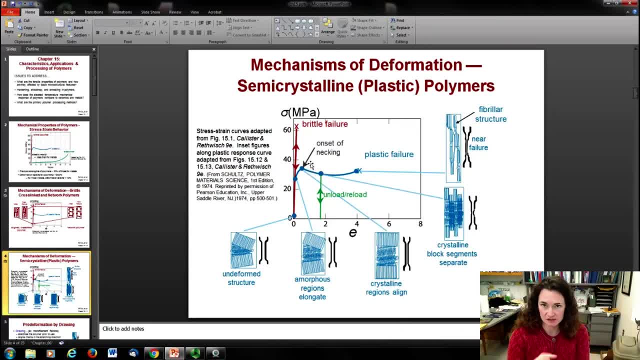 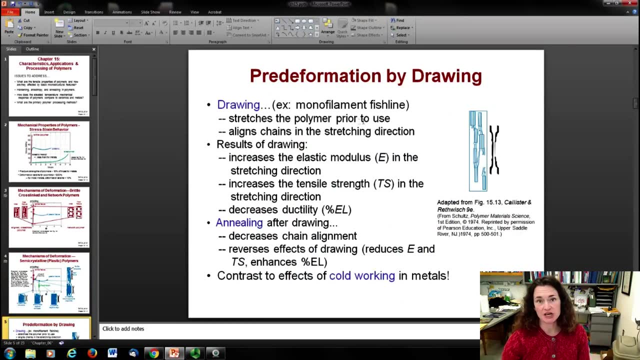 So, unlike in metals, the neck region in a polymer can substantially grow and grow, and grow, grow and that corresponds to the polymer in that region. strengthening This is often called pre-deformation by drawing. So drawing, for example, is when you take a polymer and you stretch it out into a fiber. 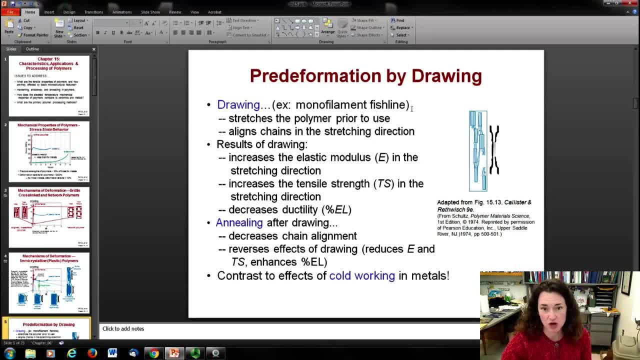 So, for example, if you're making monofilament fish line, this would be by drawing, So you stretch your polymer prior to use to align the chains in the stretching direction, and what that can do for you is increase your elastic modulus in the stretching direction. 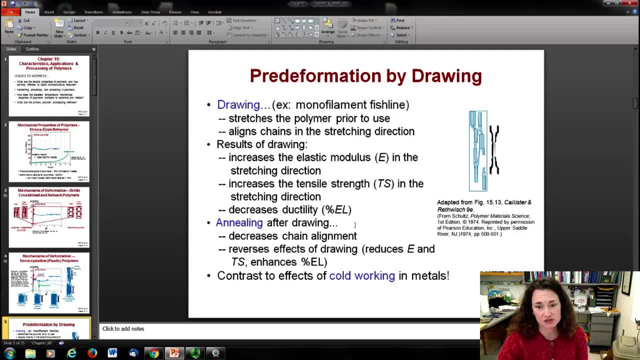 increase your tensile strength in the stretching direction but also decrease your ductility. Remember those two things are flip coin sides of each other. If you anneal it or heat it after you do that drawing, of course you're going to reverse a lot of those effects and this is very similar to the ideal cold working in metals. 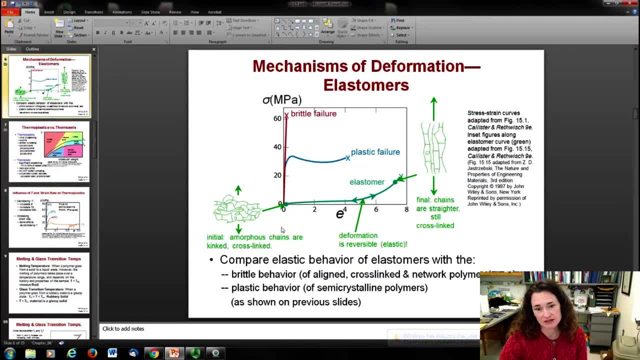 Now, if you have an elastomer, then the stress-strain curve looks very, very different. So for your brittle failure, remember you have your cross-linked polymers or your network polymers. For plastic failure, you have your semi-crystalline polymers. 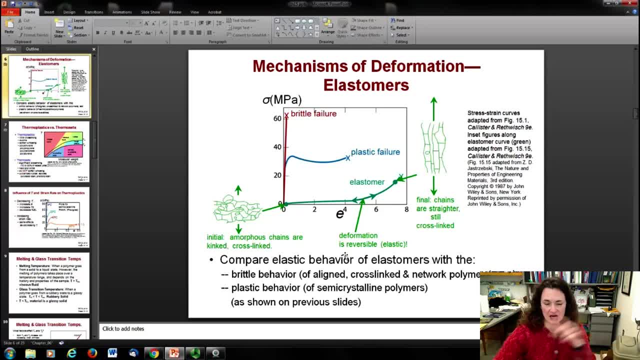 Elastomers, however, are these amorphous chains that have a lot of curving around on themselves. They could be kinked or cross-linked, And then what happens is, as you apply a stress to the material, all those kinks and twirls. 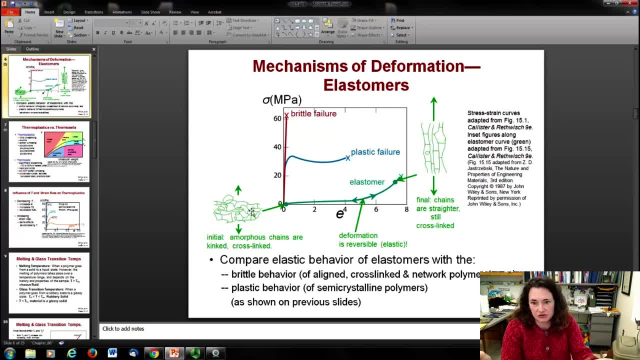 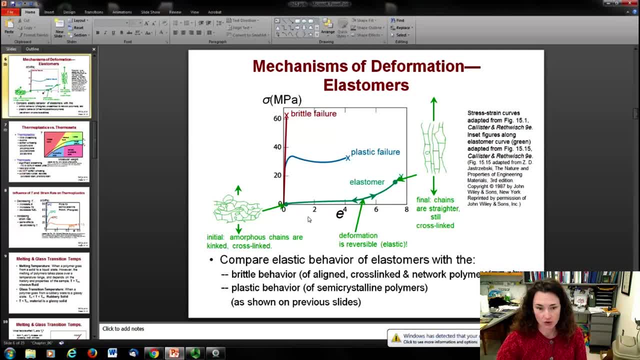 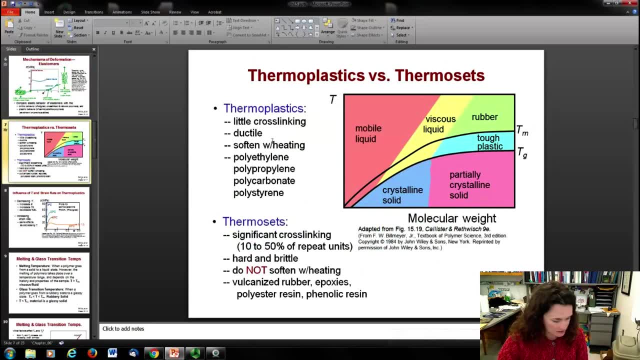 They might still be cross-linked, but they're very, very aligned. okay, There's two different kinds of plastics. They can be defined as either a thermoplastic or a thermoset, and that's because the polymers are often classified according to their behavior at high temperatures. 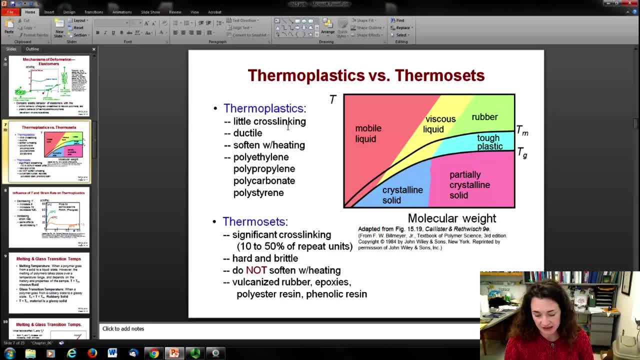 So thermoplastics: they soften when they're heated and then eventually they liquefy, and this is a reversible process. And thermoplastics are relatively soft and they're easy to recycle. However, thermoset polymers are these network polymers with extensive cross-linking, like 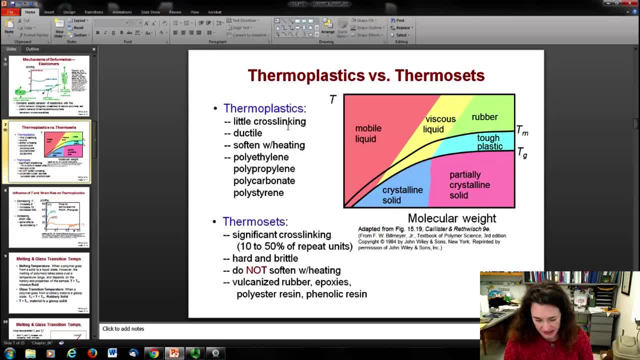 10 to 50% cross-linked, and they don't soften when they're heated, And heating to excessive temperatures will break those cross-links, but this basically destroys the polymer, And so they're not easy to recycle. So some examples of thermoplastics are polyethylene, polypropylene, polycarbonate, polystyrene. 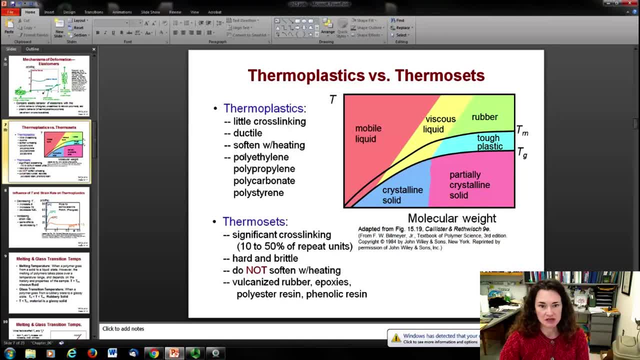 polystyrene. So that's your polyethylene might be a lot of your plastic bags, plastic bottles. polycarbonate is glassy and then polystyrene would be your packing peanuts, Your thermosets, vulcanized rubber from tires, epoxies, polyester resin and phenolic resin. 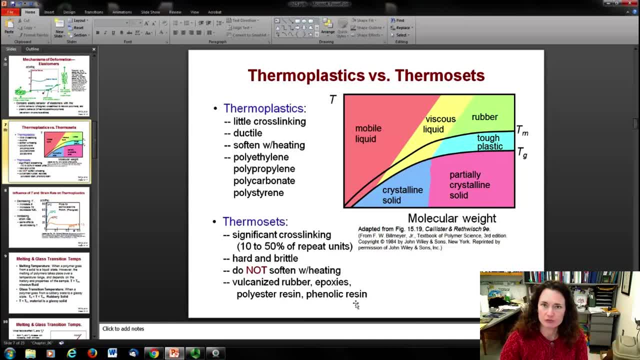 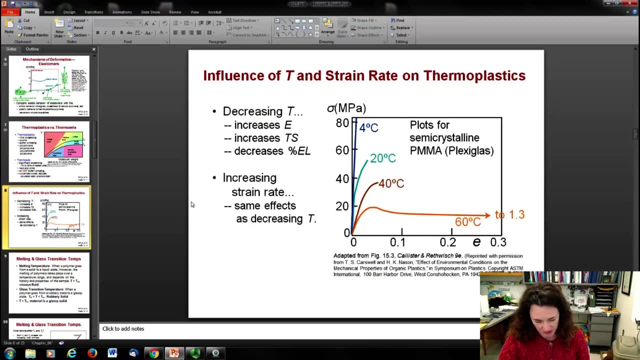 So any kind of basically setting glue that you might use that has a two-component that you mix together. those are also thermosets. Now there's a huge difference. There's a huge temperature dependence to the polymer properties. They heat up and what happens is if you decrease the temperature, you're going to increase. 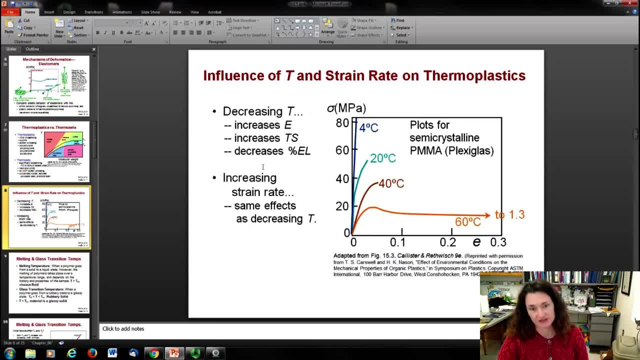 the elastic modulus increase your tensile strength and decrease your ductility. So this is shown here in some plots for semi-crystalline polymethylmethacrylate or plexiglass, and you can see what the stress strain. 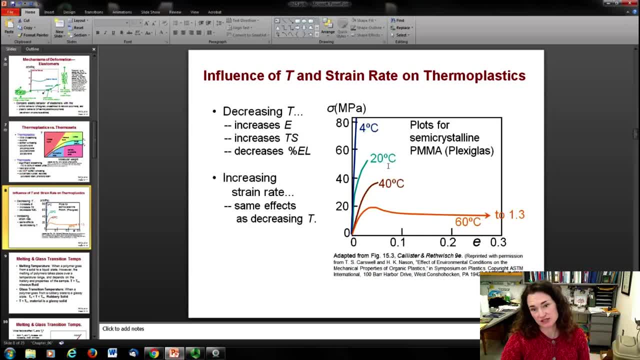 Curves look like at 4 degrees C, 20 degrees C, 40 degrees C and 60 degrees C, So you can see that they get a lot more ductile, less brittle, but also less strong as they're heated. 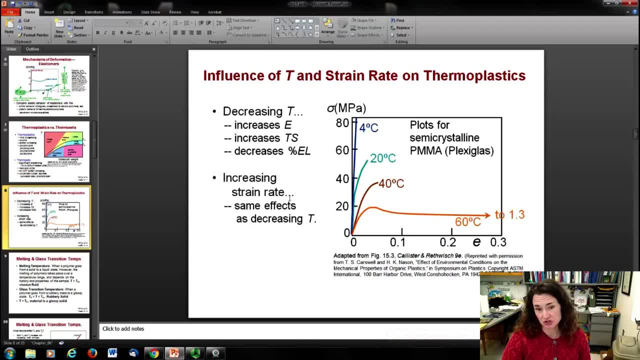 You can also see these same effects if you increase your strain rate. So if you apply force or stress faster on the material, then you can see some of the same effects, And that's because they heat up as they're deformed. But if you're strained, 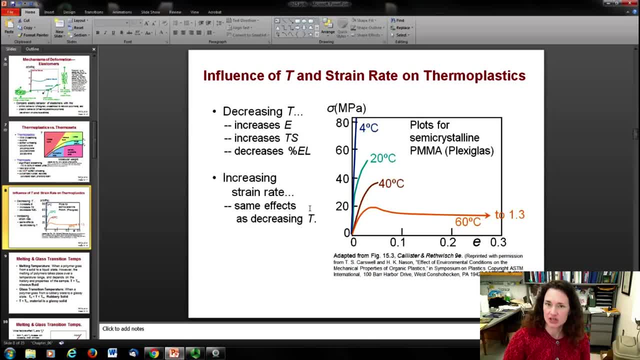 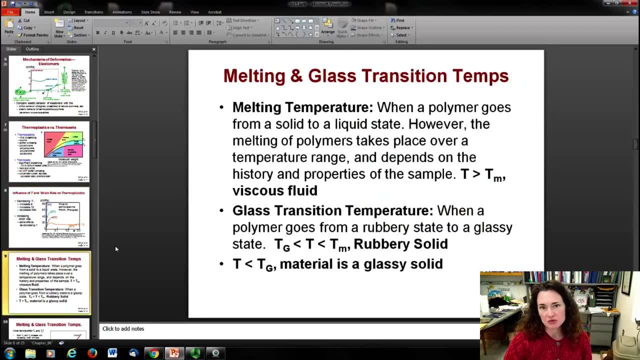 If your strain rate is too high, then they don't have time to heat up much, and so they act as a colder polymer. Sometimes, when you deal with polymers, you'll see two different temperatures given or listed in the safety data sheet. 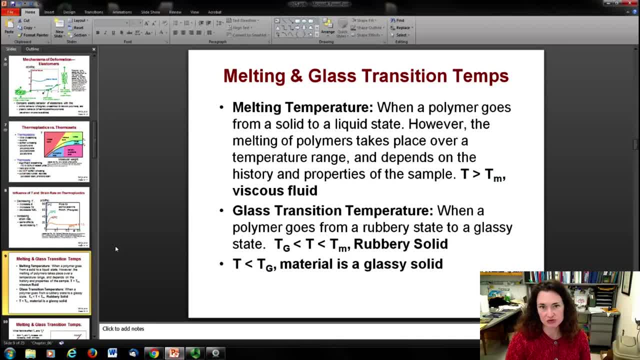 Your melting and your glass transition temperature. So these are two different temperatures and you might wonder what's going on there. Well, the melting temperature is defined as when a polymer goes from a solid to a liquid state. However, you're going to get sort of a spread in the data for that, because the melting 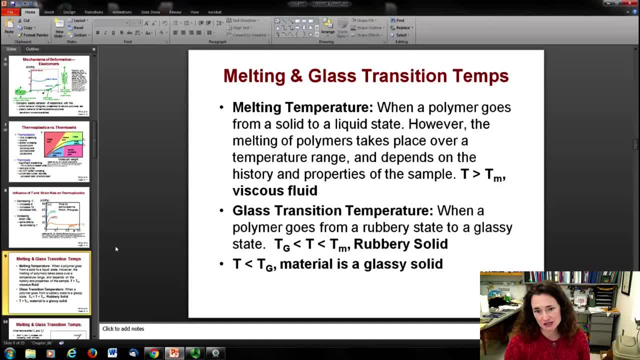 of the polymer takes place over a temperature range and is going to depend on the history and also the properties of the sample. So, for example, you might have a more heavily cross-linked polymer depending upon its history, and that might change its melting temperature. 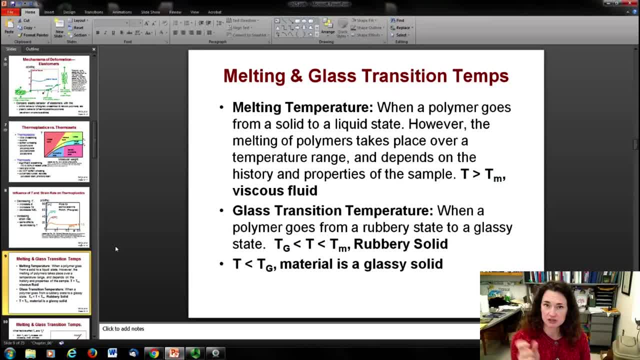 Also the molecular weight of a polymer can greatly affect and if there's some sort of spread in the molecular weight then you're going to get a melting transition temperature that might change. It might be a little different from sample to sample. If your temperature is greater than your melting temperature, you've basically got a viscous 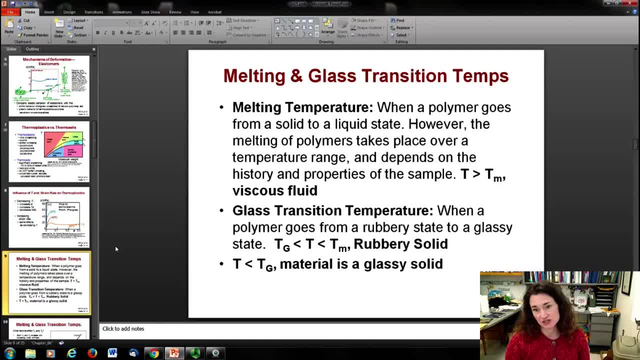 fluid. There's also defined, however, the glass transition temperature for polymers, And that's when a polymer goes from a rubbery state to a glassy state, So when a polymer is in between its glass transition temperature and its melting temperature. 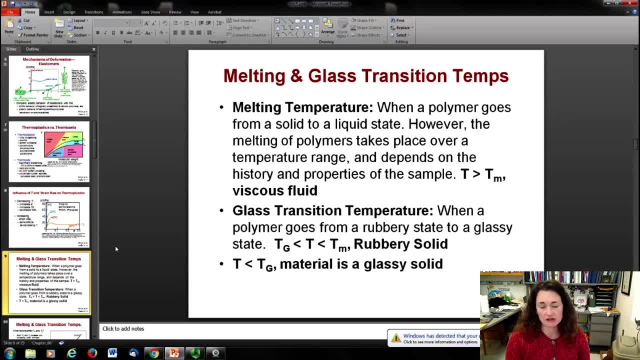 it's a rubbery solid. But if it's less than the glass transition temperature then it's a glassy solid. Now, If you have a highly crystalline polymer, then there's not a very large range temperature difference between the glassy and the glass transition temperature and the melting temperature. 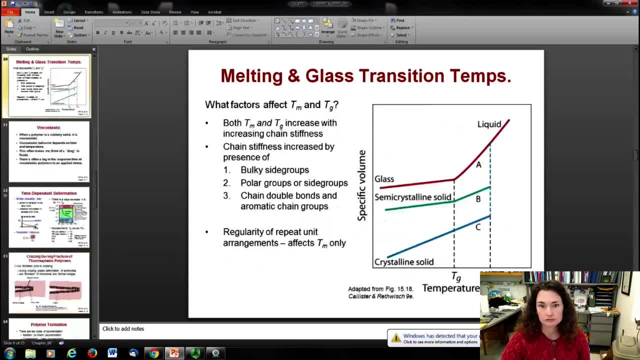 so they come together. So what factors can affect the melting temperature and the glass transition temperature? Well, both of these things increase with increasing chain stiffness, and the chain stiffness can be increased if you have bulky side groups, if you have polar groups or side groups, or 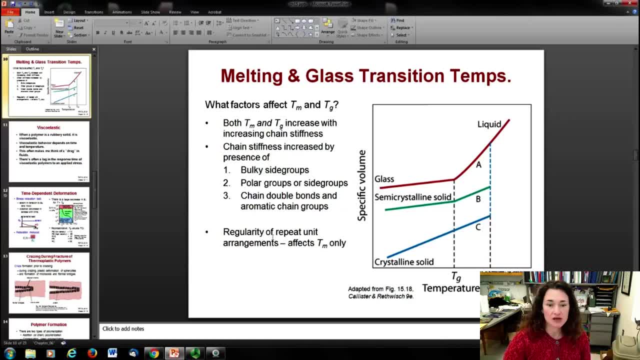 if you have double bonds and aromatic groups, And the regularity of the repeat unit arrangements affects only the melting transition temperature, And so you can see that for a crystalline solid you can see that there's these different behavior with temperature. You have sort of a straight line behavior for the density or specific volume for crystalline. 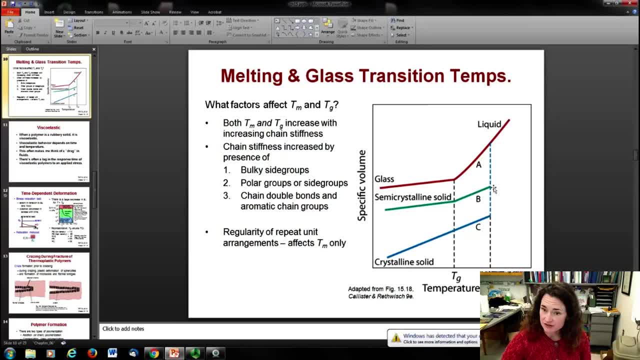 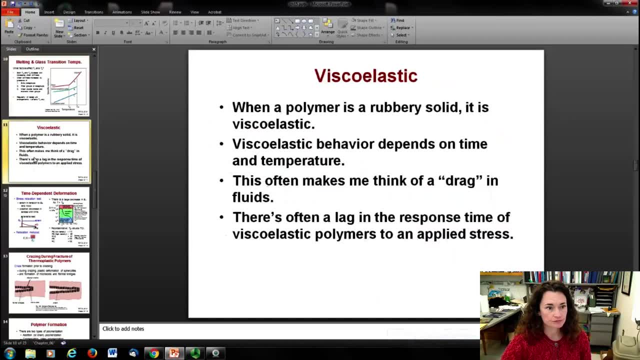 solids. For a semi-crystalline solid you can see kind of two different slopes there, And for a glassy polymer you can see a more dramatic change in the slope. You might also hear the term viscoelastic applied to polymers. 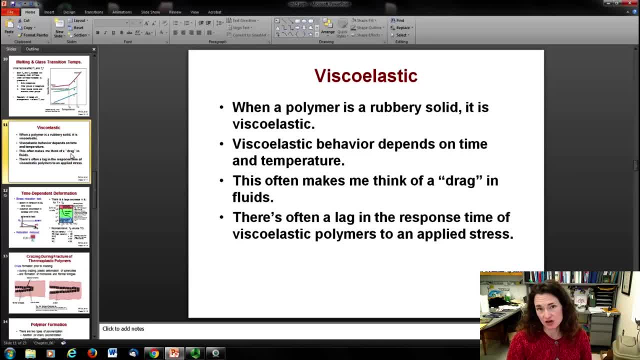 When a polymer is a rubbery solid it's called viscoelastic And the viscoelastic behavior can depend upon time and the temperature And this kind of makes me think of drag in fluids. The time dependence kind of makes me think of a drag. 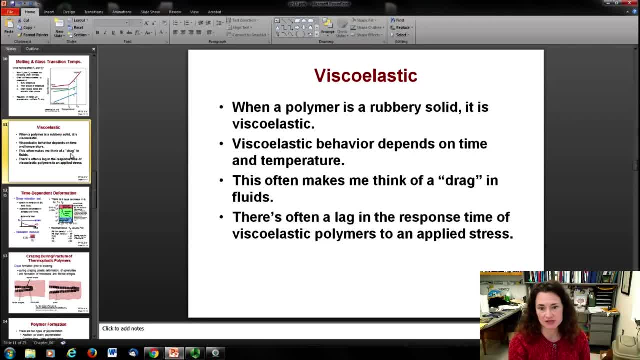 And that's typified by. there's often a lag in the response time of viscoelastic polymers to an applied stress. So you'll pull on it and then it kind of slowly deforms. It doesn't deform right away, but slowly deforms. 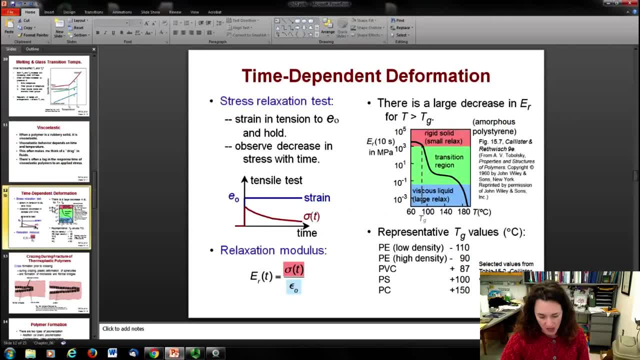 There's a lag- sort of a phase shift if you will- And this can be quantified with these stress relaxation tests. So, since there's that lag in the response time to an applied stress, to measure this property you apply the stress relaxation test. 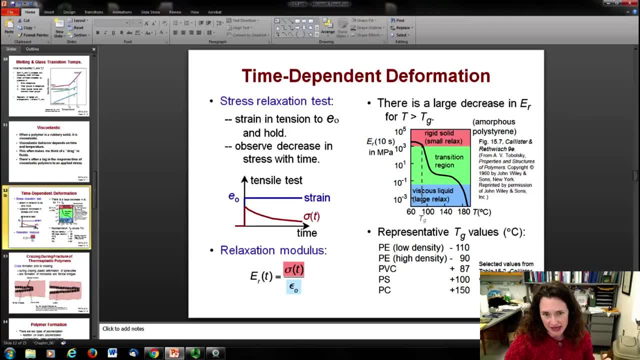 And here what you do is you have a strain in the tension and you pull it to a certain strain and then you hold it, And then what you do is you measure the applied stress that is required to maintain this strain And you can watch that applied stress decrease with time. 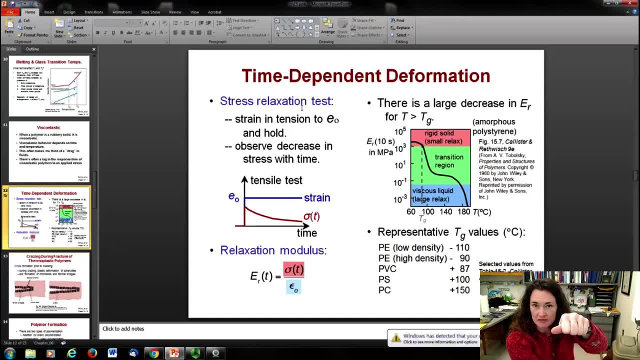 So you can put it in a machine, you can give it a pull And then you can try and maintain that same displacement while measuring the force that's required to maintain that displacement, if that makes sense, And you can watch that stress fall off with time. 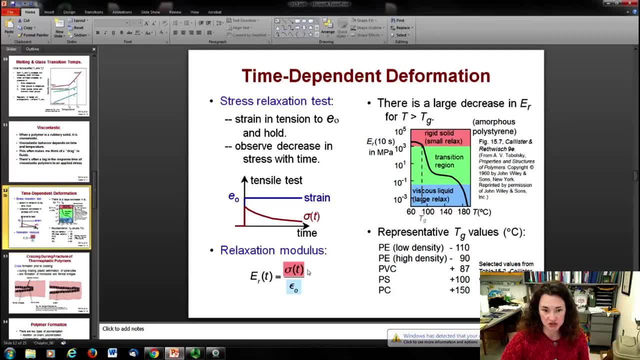 And this can be quantified by a relaxation modulus. It's shown here in this equation, sigma of T over that strain that you're applying that set strain And you can see that there's a large decrease in the relaxation modulus when the temperature. 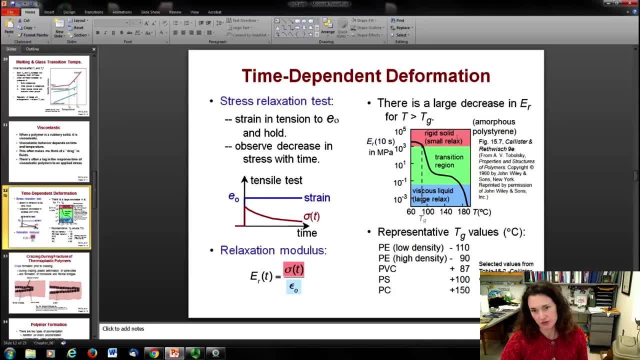 is greater than that glass transition temperature, which makes sense. And here's a plot that shows how the relaxation modulus changes with respect to temperature here, ranging from 60 to 180 degrees Celsius for this amorphous polystyrene material. And you can see that for temperature it changes from 60 to 180 degrees Celsius for this amorphous polystyrene material. 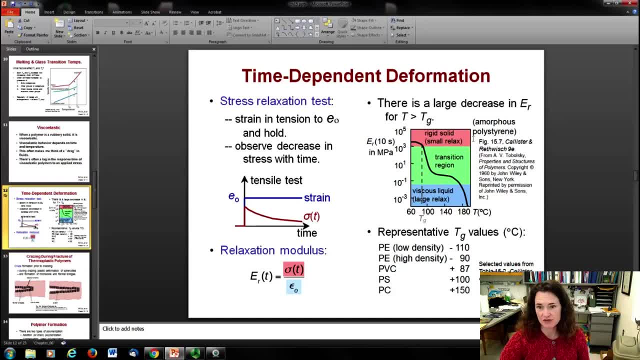 And if you look at this diagram, you can see the temperature changes here and you can see basically when it's less than the glass transition temperature. You've got basically a rigid solid that only has that small relaxation time And then there's a transition region and then it starts to act like a more viscous 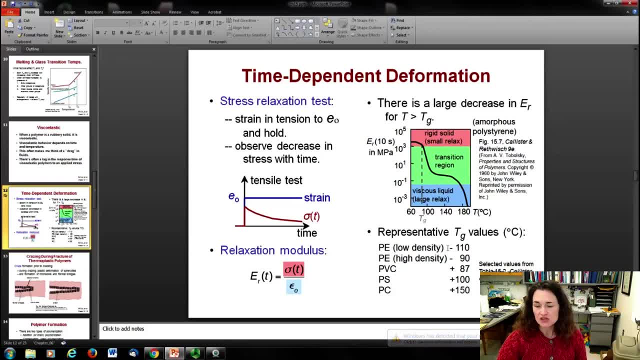 fluid with a large relaxation time. So here's some representative glass transition temperature values in Celsius for various polymers. For low density polyethylene and high density polyethylene you have low temperatures, minus 110, minus 90 degrees Celsius Celsius. For PVC it's a higher temperature: 87 degrees Celsius. Polystyrene: 100 degrees. 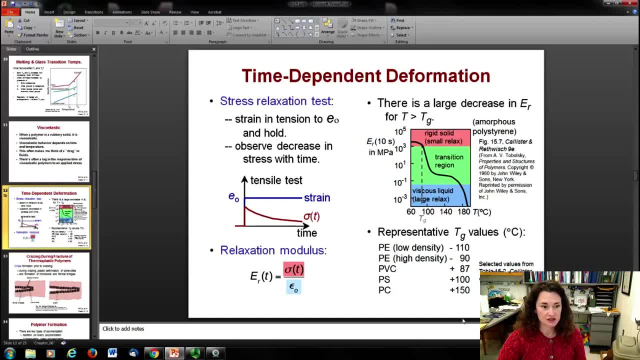 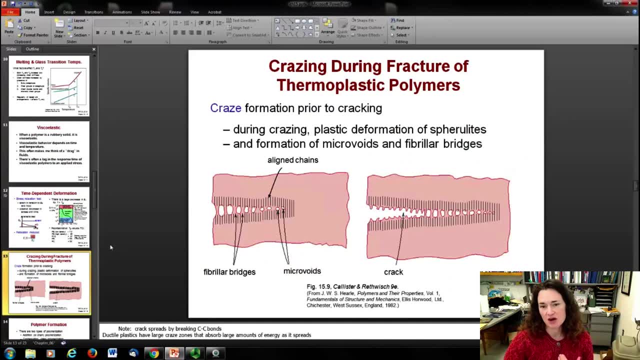 Celsius And polycarbonate 150 degrees Celsius, So there's a large temperature range there. For thermoplastic polymers, you often see a phenomenon that's called crazing during fracture, And what that is is you can get a craze forming in the polymer prior to cracking. 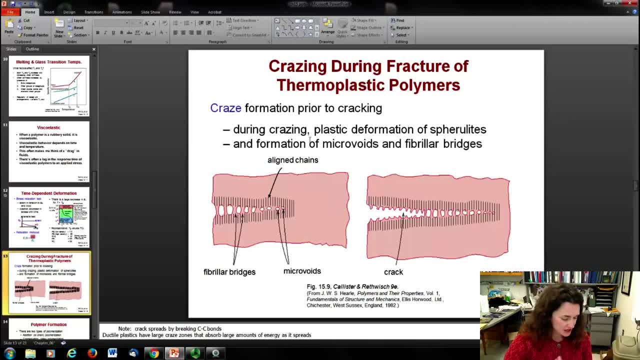 Okay. So what's going on with this is just like in metals: defects, cracks or sharp corners in your material are often points of initiation for your failure. So crazing is a phenomenon that precedes fracture in thermoplastic polymers, And it's localized. 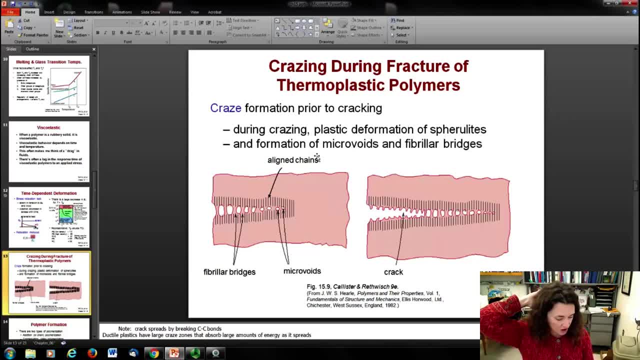 plastic deformation, which leads to these small and interconnected microvoids that are shown here in the regions, And then these little bridges, these little fibrillar bridges, form. They form between the microvoids, And that is because the chains are becoming aligned. 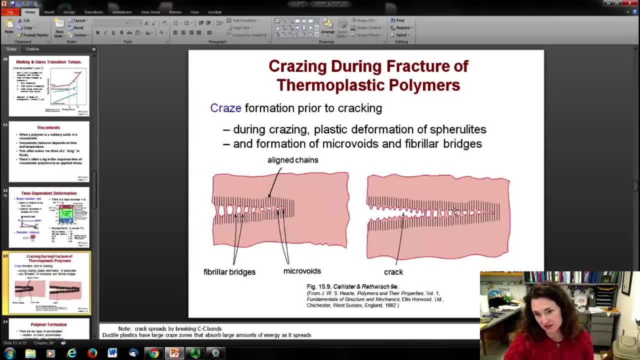 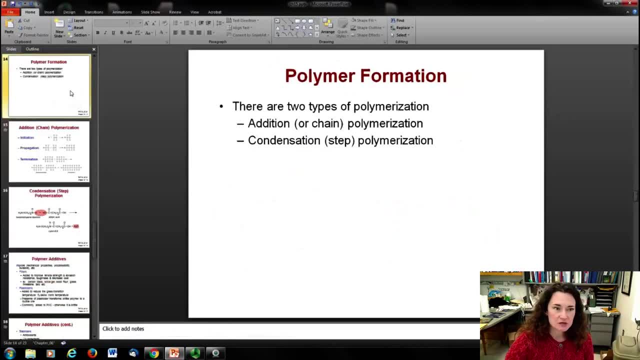 in that region And then that propagates through as the crack when failure is completed. We talked a little bit shifting gears. we already talked a little bit about polymer formation in an earlier chapter, But just to reiterate on that, there's two types of 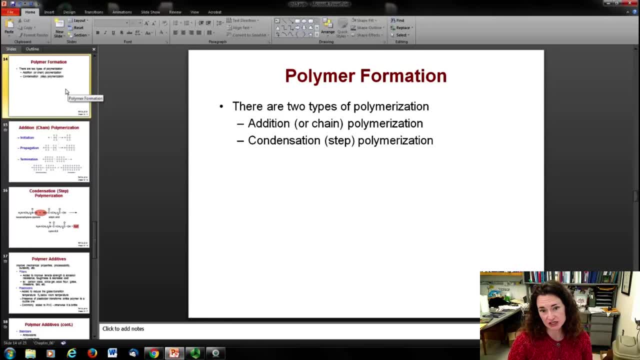 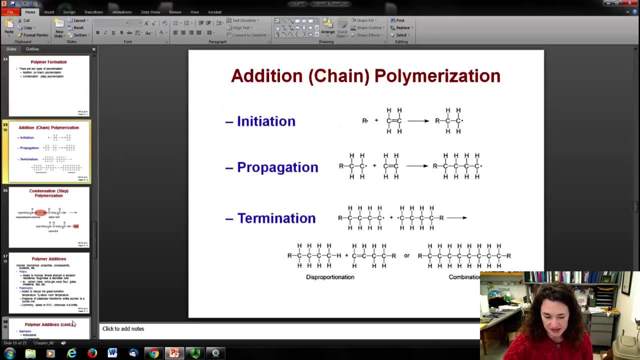 polymerization. There's the addition or chain polymerization, And then there's a condensation or a step polymerization. So when you're synthesizing these large molecules, your monomers, they usually come from coal, oil, natural gas and petroleum products. 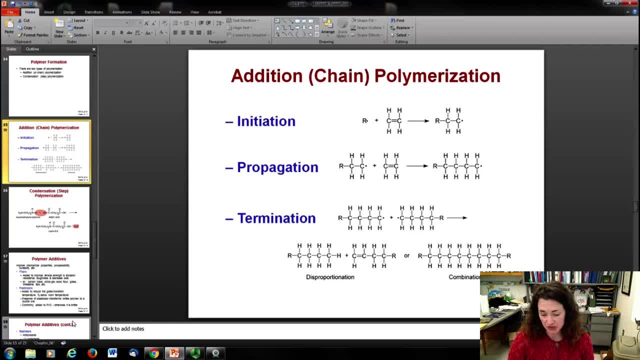 And, in addition to polymerization, what you do is you take a monomer unit and attach it one by one, And there's three steps to that, Of course. initiation is when you introduce that free radical And the free radical breaks some of the intercarbon bonds. 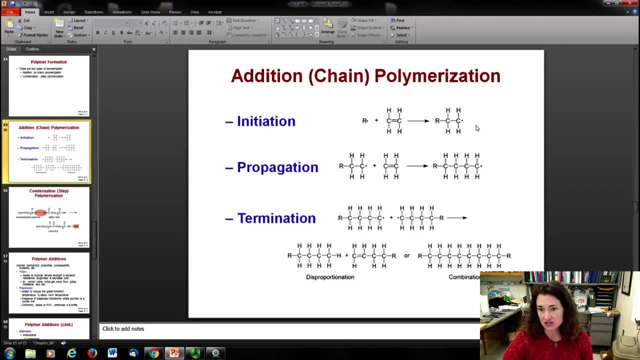 So you take the intercarbon bonds in your monomer unit and then attaches And when that breaks, this carbon over here has a free dangling bond And then that continues the reaction into the propagation step. The chain growth's rapid. It only takes about 10 to the minus 2 to 10 to the minus 3 seconds. 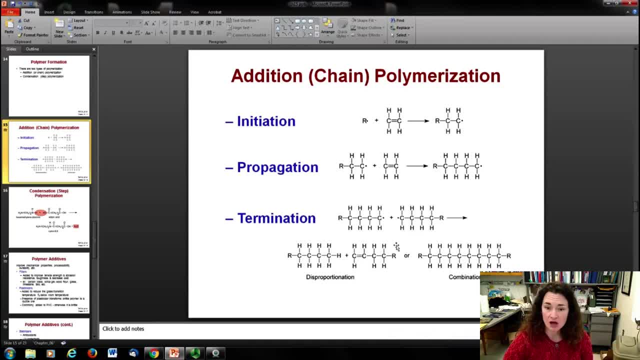 to form a 1,000 repeat unit chain And then, when you want to stop the reaction, you can terminate it one of two ways: You can either introduce a green That will bond with the free radical on one end and stop it that way, Or you can get the 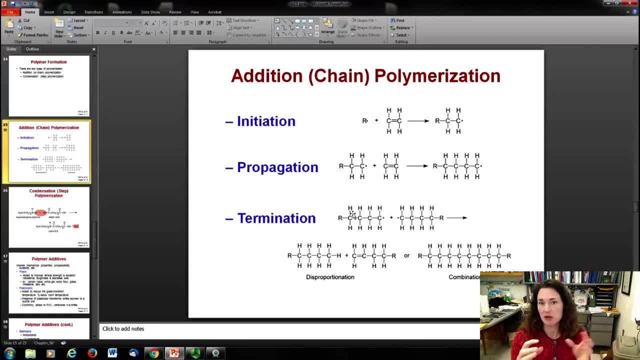 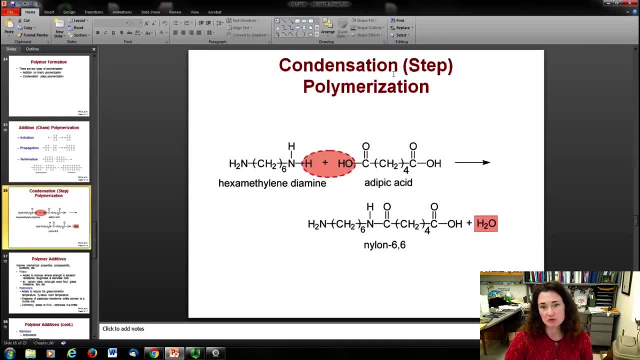 chains to hook together to each other and kind of combine to form one big polymer unit. There's another type of polymerization where you're hooking together two dissimilar materials, kind of A, B, A, B, A, B, like that. This is similar to what we're going to do in a. 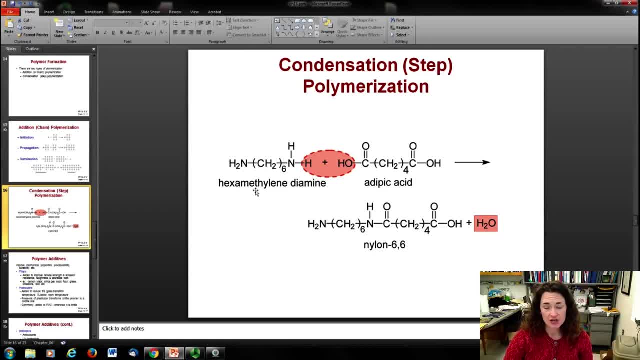 lab to make nylon 6.. have these two materials, you break the bonds there and you hook them to one another And then the reaction can just continue. So you have this hexamethylene diamine that hooks up to this acid here, And then on the other side you can get another hexamethylene diamine and hook it up there. 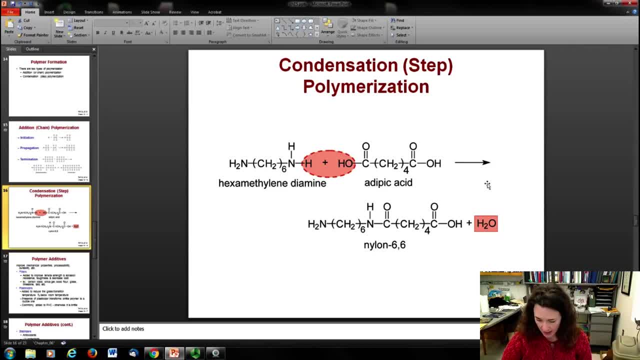 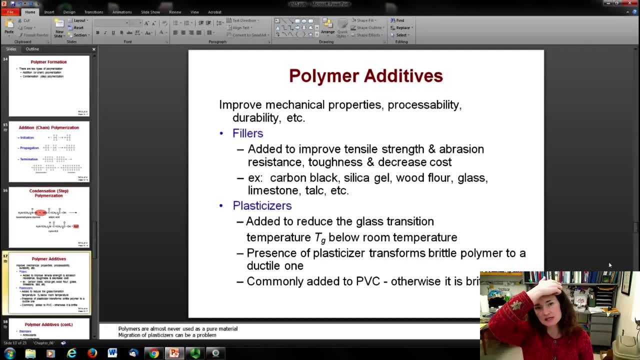 and so on and so forth And the reaction proceeds in that way. But anyway it's a chemical reaction between two different species. Lots of times in factories they'll want to add additives, polymer additives, And the additives can improve the mechanical properties, processability. 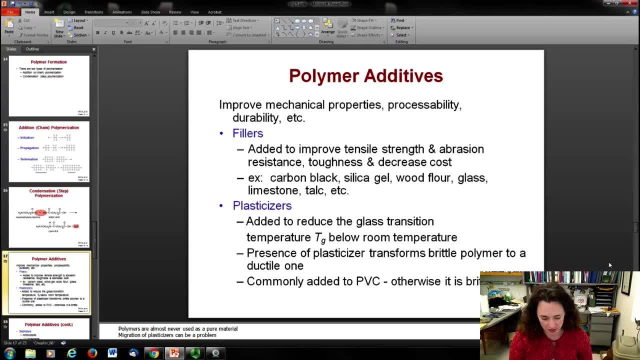 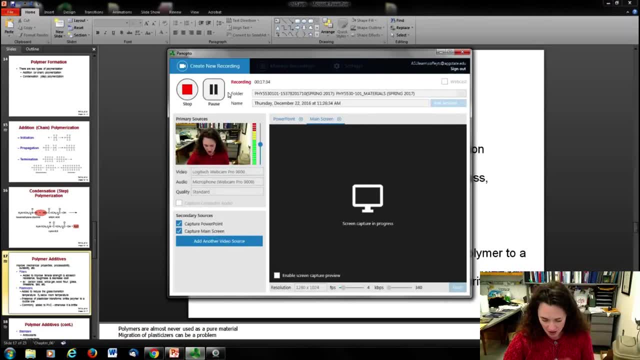 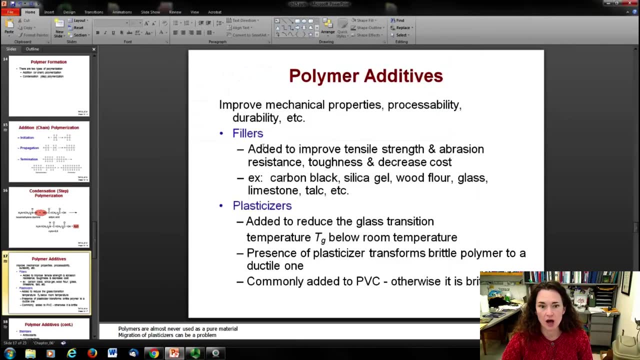 durability of the polymers, among other properties. So there's a couple of main ones. Pardon me, Sorry about that. Okay, so the additives, they form these composite materials for fillers. So you can see here fillers are added to improve the tensile strength and the abrasion resistance toughness and to 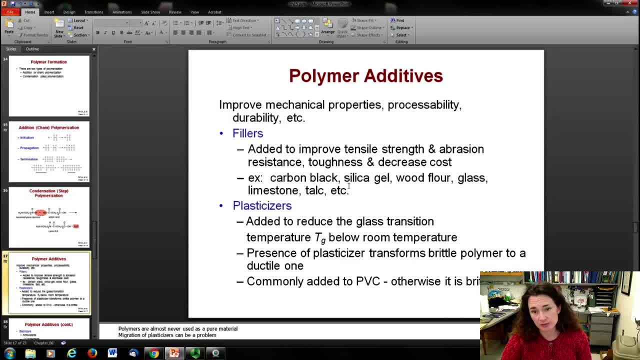 decrease cost. So, for example, you might add carbon, black silica, gel, wood flour, glass, limestone, talc or a lot of other things to improve those properties, And when you do that, you're basically forming a composite material. On the other hand, plasticizers are generally liquids. 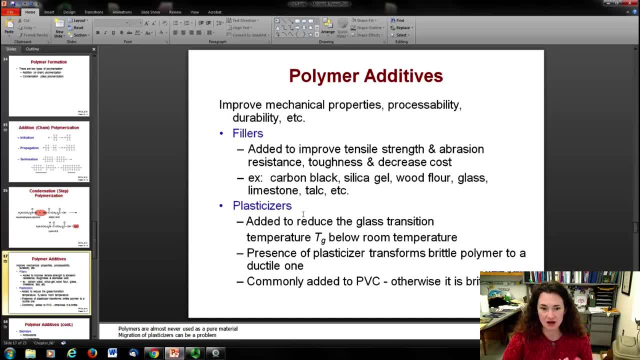 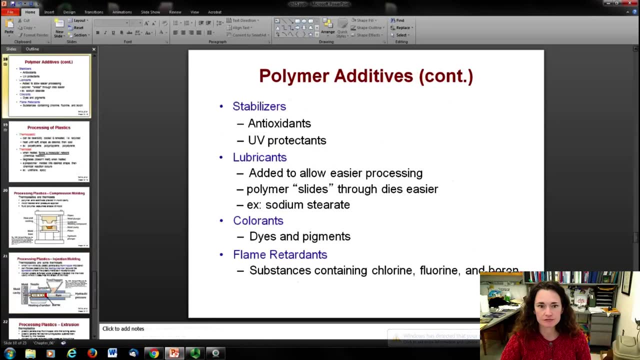 with low molecular weights And they're often added to reduce the glass transition temperature below room temperature or transform a brittle material into a more ductile material, And this is commonly added to PVC. Otherwise it's really brittle and it fractures very easy. You can also 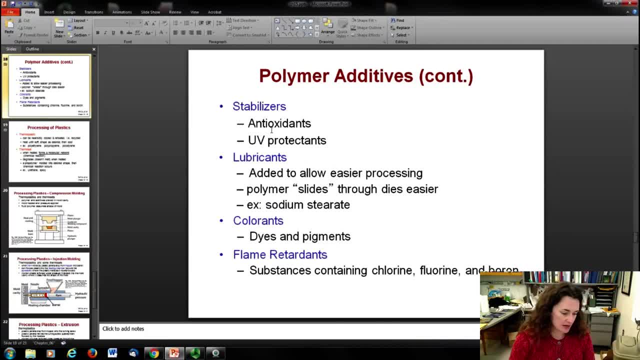 add stabilizers And the stabilizers might protect it from degradation due to oxygen or ultraviolet radiation. You can add lubricants to allow easier processing. If you have a high coefficient of friction, for example in between your polymer and the material, you can add lubricants to allow easier. 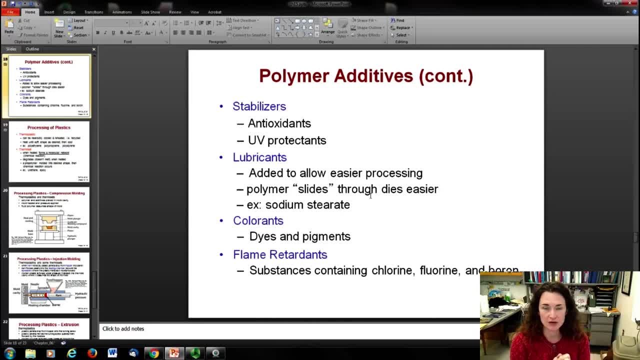 sliding And some of the rollers and the dyes that you might use in a processing plant. then you might want to add a lubricant to add easier sliding. An example of that is sodium stearate. You might want to color your polymer, make it pretty for toys or whatever other application, And then you add dyes. 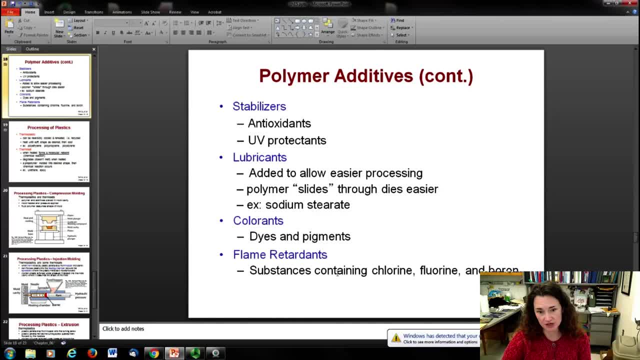 and pigments to it, And you might also want to add flame retardants. These are usually substances that contain chlorine, fluorine and boron, And of course, you might want to do that to reduce the flammability of your material. 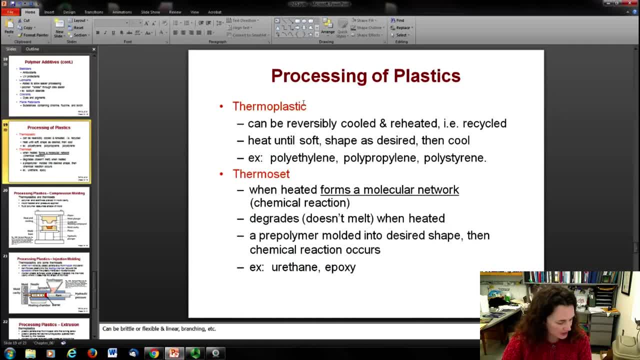 The processing of plastics. Remember, your thermoplastics can be reversibly cooled and heated, They can be recycled, And there you can also heat them until they're soft and then shape them as you desire and then cool them. And of course these are the polyethylene, polypropylene, polystyrene, polycarbonate. 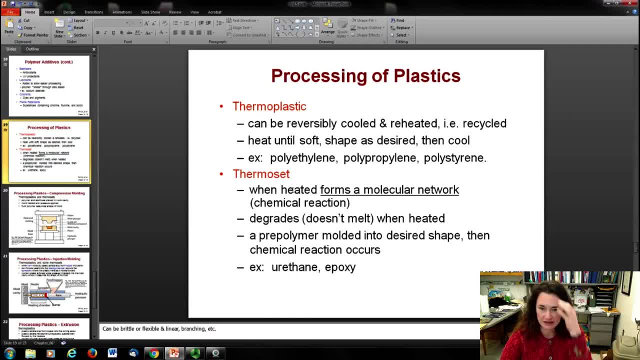 materials, Your thermoset polymers. however, when they're heated, they form a network. It's a chemical reaction, kind of like mixing the two materials together in an epoxy, And it degrades. It doesn't melt when it's heated. So what you have to do there is you have to have a pre-polymer that's molded. 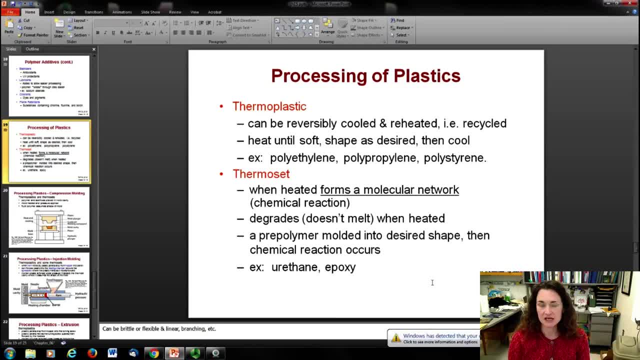 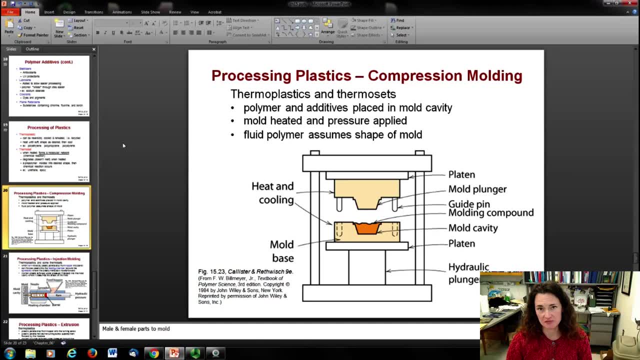 into a desired shape and then have that chemically react, And for example they're urethanes or epoxies. I have some videos for you to watch that are from other sources. I've listed the links on our course web page And they're a lot of fun watching these things as they go through the factory and how it's. 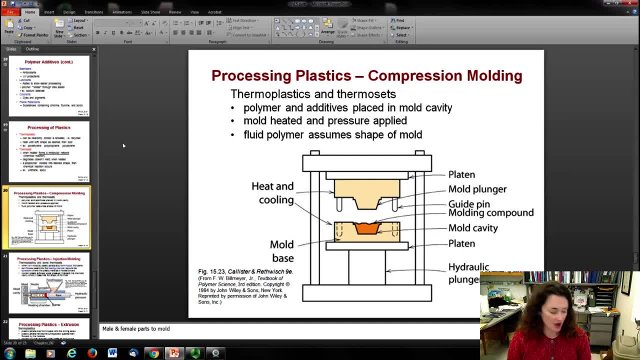 actually done. But to just kind of briefly explain how polymers are processed: In processing plastics you can do several different techniques. One is compression molding, And these are done for thermoplastics and thermosets, And in that you take the polymer and its additives. 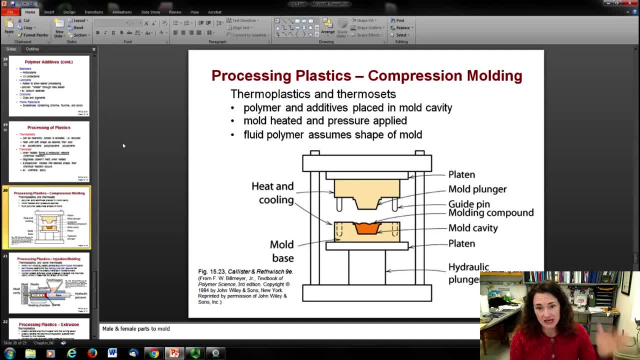 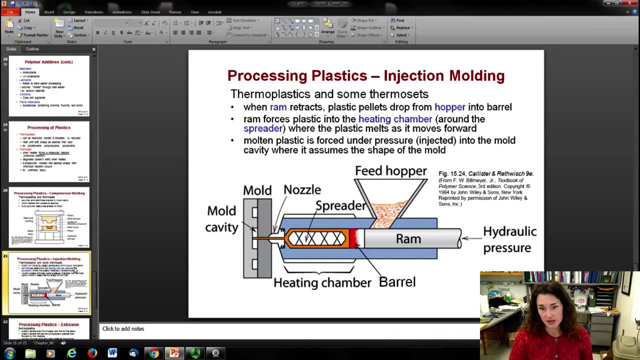 and you put it in a mold cavity And then the mold's heated and it's brought together and pressure's applied And then your polymer kind of assumes the shape of the mold. So that's compression molding. You can also do injection molding. This is done with thermoplastics and some thermosets, And so what? 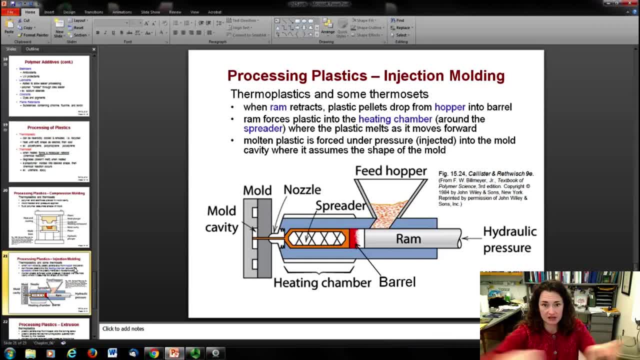 you do. there is you have a ram that gets pulled back And then plastic pellets from your hopper drop into the barrel And then you push your ram in And that forces the plastic into a heating chamber around your spreader where the plastic melts as it moves forward, And then that molten plastic is forced under pressure. 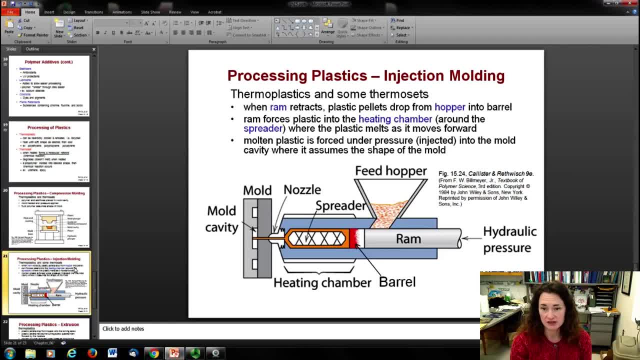 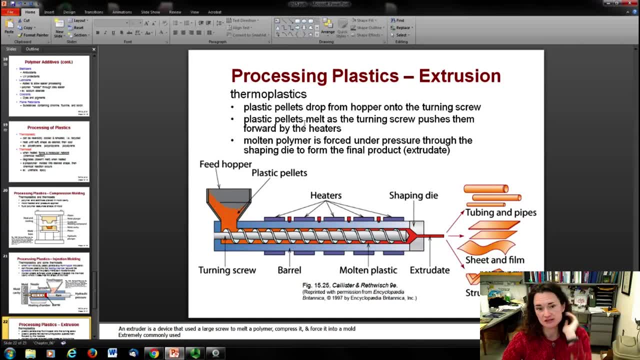 into a cavity And it assumes the shape of the mold. They do this with Legos. You can also use extrusion. This is done with thermoplastics And it's similar. You have a hopper with plastic pellets that drop from the hopper into a turning screw. 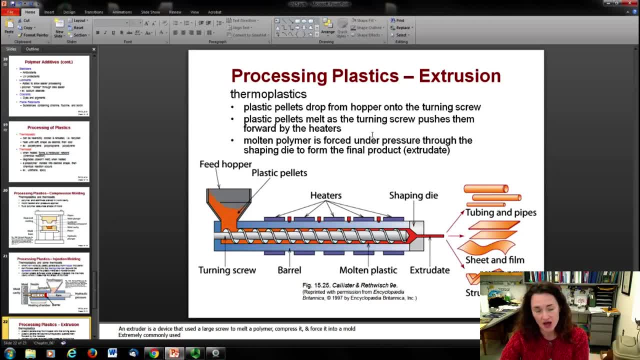 And then the pellets melt as the turning screw pushes them forward, And then the molten plastic is forced under pressure through a shaping die to form a final product And you use this if you want to do tubing, pipes, sheets or structural parts.